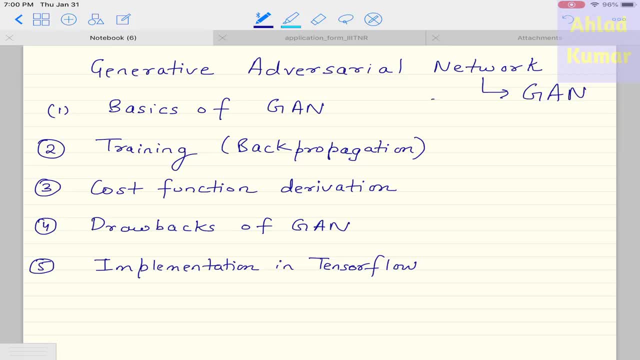 In the first lecture. what we will do is we will discuss the basics of GAN and the training process that is involved in this GAN, And by training I mean to say how you will train the GAN during the back propagation process. So we will discuss the basic concepts of these in our first lecture. 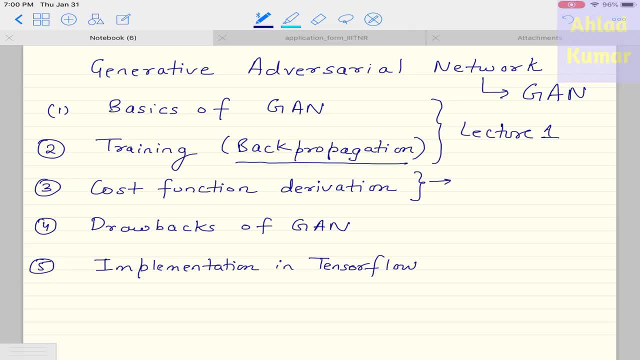 In the second lecture, what we will do is we will derive the cost function of GAN in greater details and our target is to understand each part of that derivation effectively. And in the third lecture, what we will do is we will do the understanding of the drawbacks of GAN, that what drawbacks the GAN has and how to overcome it if it is possible. 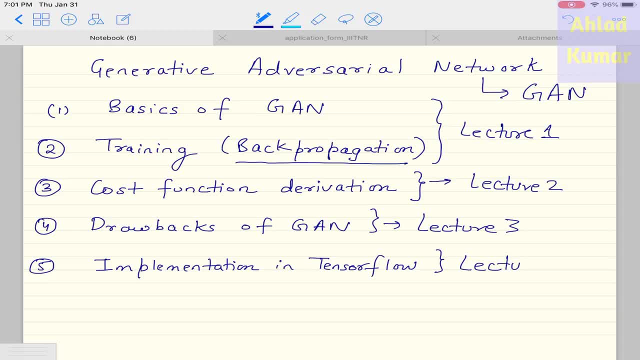 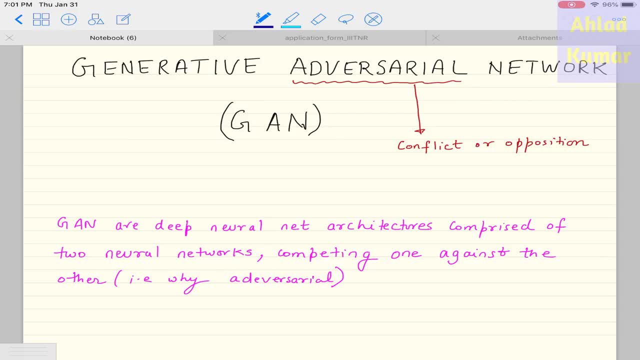 And in the last lecture, what we will do is we will implement the GAN in tensor flow. So, without wasting any time, let's start understanding the concept of GAN. So, as the name suggests, we have these 3 terms: that is generative, one is adversarial, another one is network. So this GAN composed of 3 different terms. 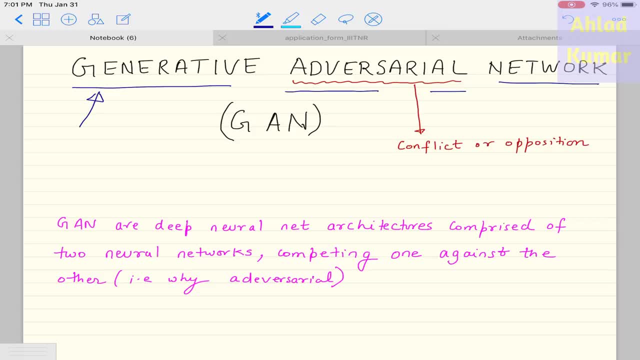 We can understand that. what generative means? by our previous lectures, if you have seen, for variational autoencoders, in which we generated some probability distribution function that mimicked the original probability distribution function of the MNIST data. So we will discuss this in more detail as we will move forward. 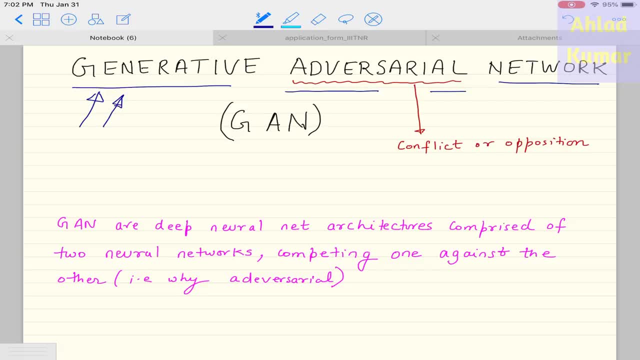 So by generative we mean to say we will generate some probability distribution which becomes close to the original data that we want to approximate By saying that it's adversarial. So adversarial means in English dictionary adversarial means conflict or opposition. So there will be 2 networks, which we call them as discriminator and generator. 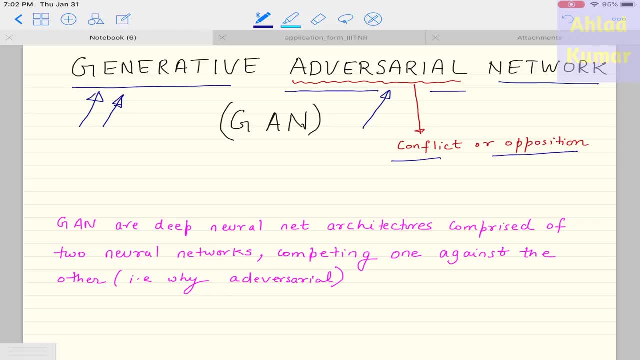 So these 2 neural networks will be fighting against each other in order to learn the probability distribution function. So adversarial comes because of that reason. So now we will go through the definition, And the definition is that GANs are deep neural net architectures comprising of 2 neural networks competing against each other. 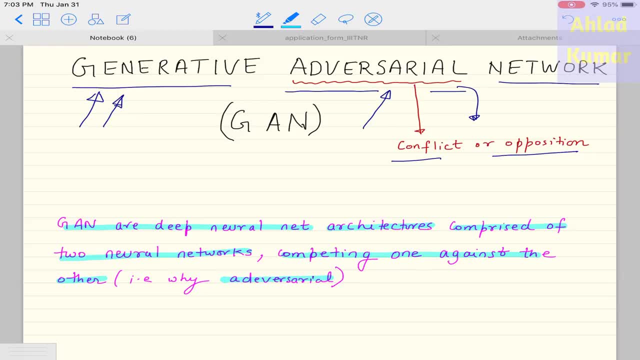 That is why this adversarial comes And the adversarial term comes into play. And by network we mean to say they are the deep neural networks or the CNN networks or simple vanilla networks. So by understanding these 3 terms, that is, generative, adversarial and network terms. 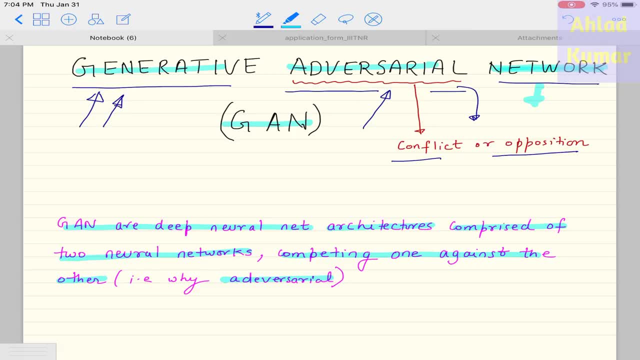 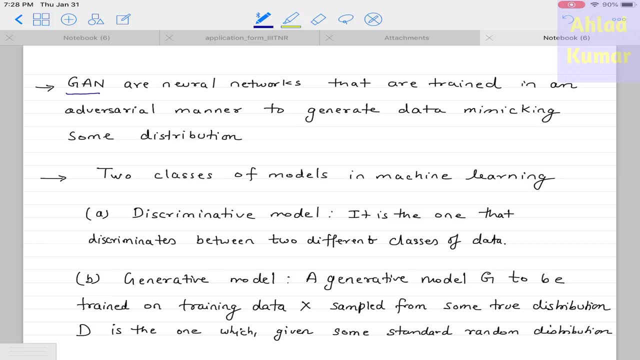 Now we are in good shape to understand what GANs are actually all about. So let us see. what are generative adversarial networks? Basically, generative adversarial networks are simple neural networks that are trained in an adversarial manner, So they are generative adversarial networks. 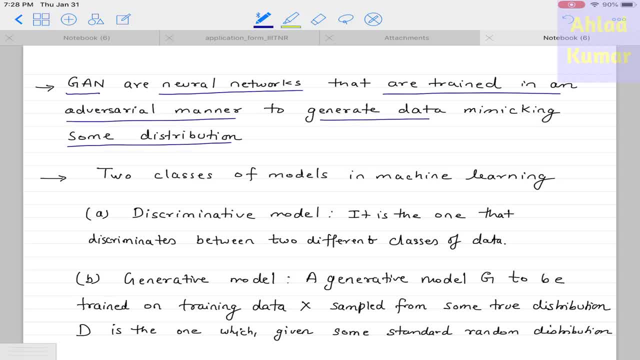 And they are trained to generate data that mimics the distribution that we want to actually approximate. We will see what that is in the coming slides, But for now you can understand that this is the main objective of generative adversarial networks, That is, to generate some new data that mimics the distribution which we are trying to approximate. 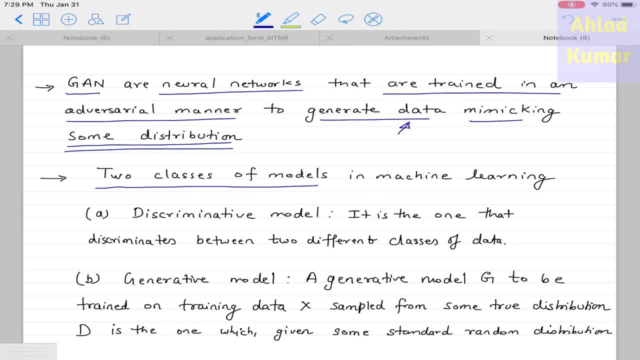 So let us move further. So there are basically 2 classes of models in machine learning which are important. The one is the discriminative model And the second one is the generative models. So let us discuss each of them one by one. 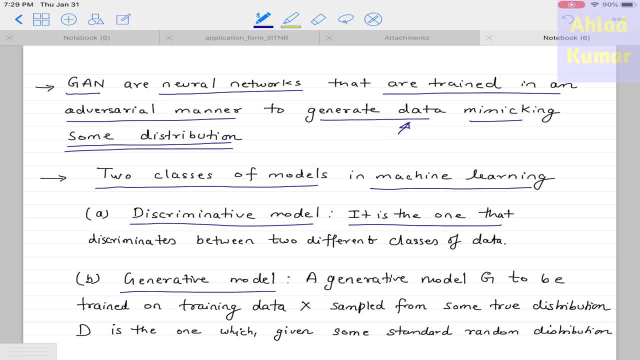 So what are discriminative models? They are basically the one that discriminates between 2 different classes of data. So, for example, if you want to classify whether the face is fake or not, Then it is done through the discriminative model And the output of this discriminative model will be 0 if it is fake. 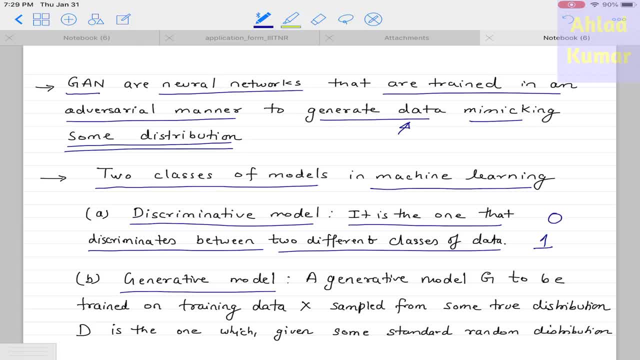 And 1 if it is not a fake face, That is, it is a real face. So all these discriminative models fall in the category of classification problem, And we have seen a lot of these problems in machine learning. So the next models that are important are generative models. 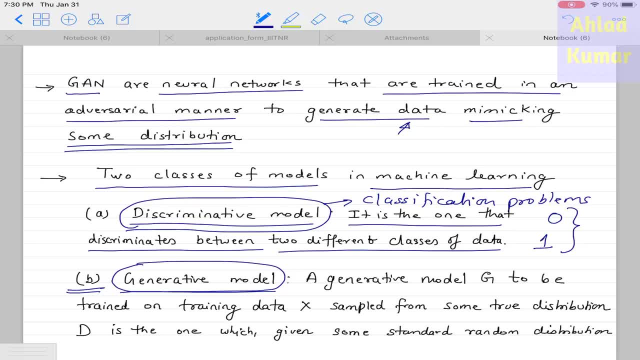 They are different categories as compared to the discriminative models. And what are they? A generative model, which is basically represented by capital G, Which has to be trained on the training data X Sampled from some true distribution. D Is the one. 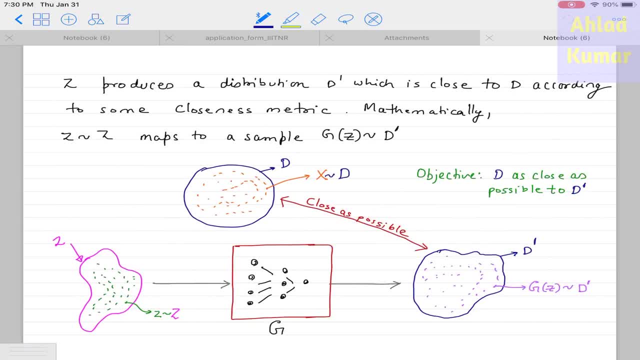 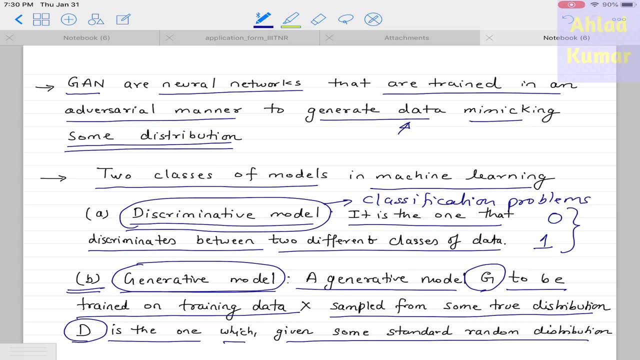 Which, given some random distribution Z, Produces a distribution D hat Which is as close to D according to some closeness metric. I can understand that these statements are bit confusing to you, So let's discuss each of these lines in detail by showing you all these things in a pictorial representation. 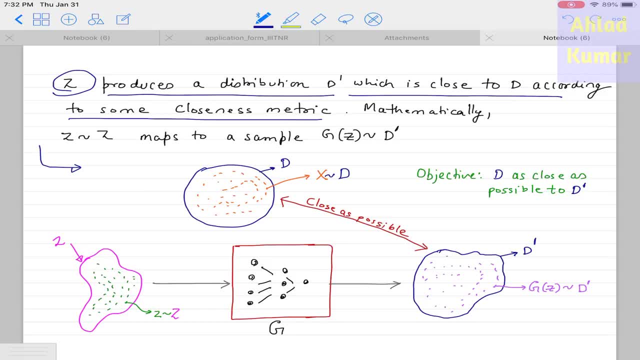 So let us explain this pictorially, As you can see that we are representing the original distribution as a circle, And this original distribution is represented as capital D And all the data points inside that are represented by capital X And these X. you can take, for example, MNIST data set. 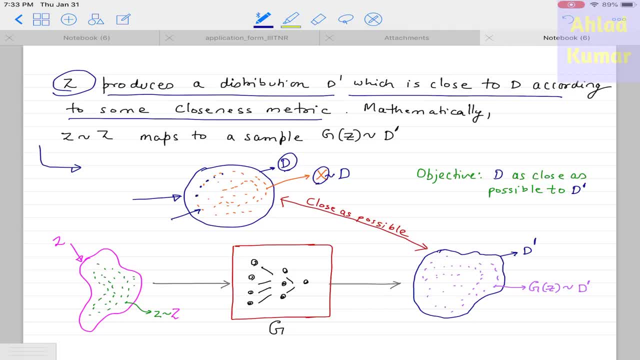 All these orange points are MNIST data set And these data sets forms a distribution, capital D, which is unknown to us. So you can think like you have this data set of MNIST numbers And you cannot tell what kind of distribution this MNIST data set is. 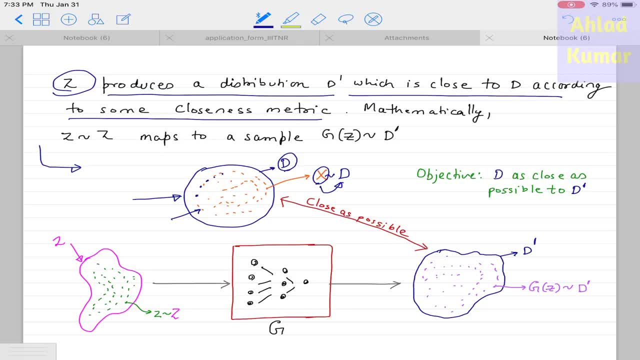 What kind of distribution this MNIST data set numbers are forming. So that's why we are representing the distribution of this MNIST data samples as capital D. So what we want from our generator is to approximate this D And come as close as possible to this capital D. 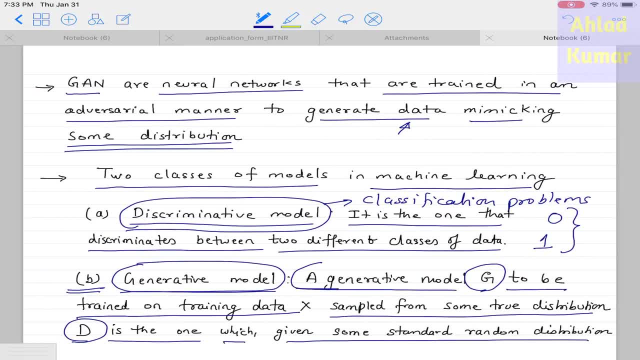 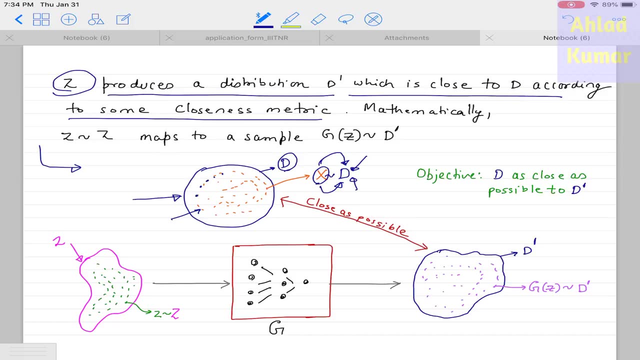 So that is what is written over here. That is a generative model. G Has to be trained on the training data X. That is basically sampled from some true distribution D. So that is, X is basically sampled from this true distribution D And our model has to be trained on that. 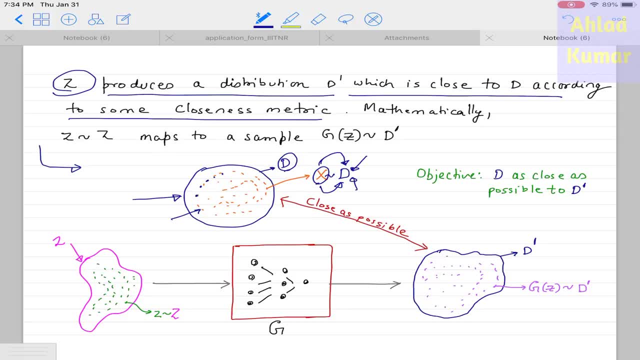 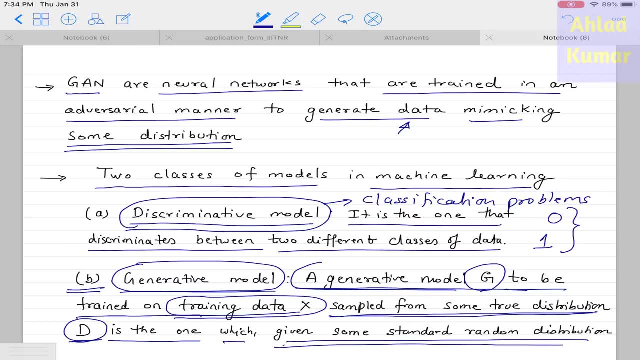 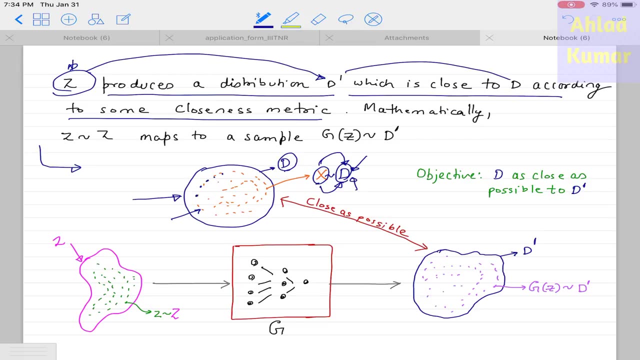 So that it produces another distribution which is as close to D. And how we will do that? We will do that by given some standard random distribution, Z, And transferring this random distribution to D hat, Which is as close as possible to D. So let's see what it means in terms of pictogram. 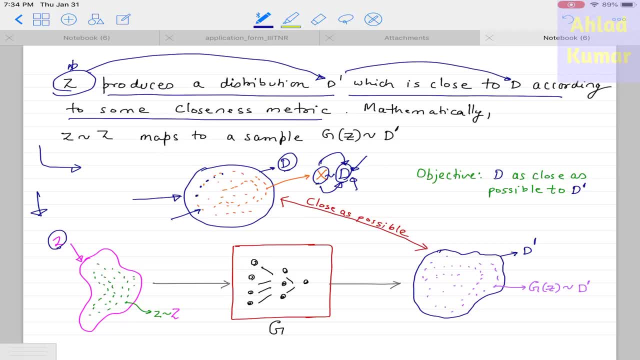 Pictorial representation. Here we have this capital Z as the random distribution. So the target of the generator model, which is represented as G over here, Is to convert this random distribution, capital Z, into D hat, And the D hat should be as close as possible to D. 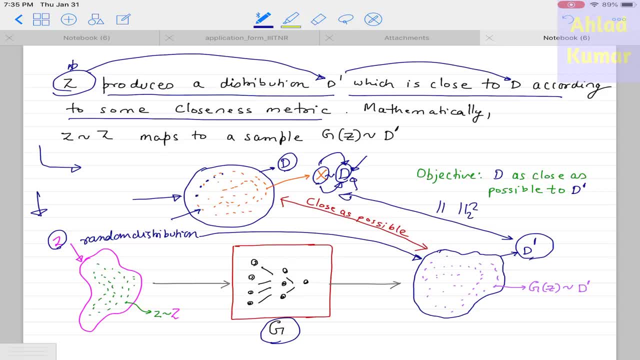 In terms of some metric May be L2 norm or L1 norm, So we want our D hat to be as close to D And this generator G is basically A feed forward neural network or deep neural network, Or it can be CNN. 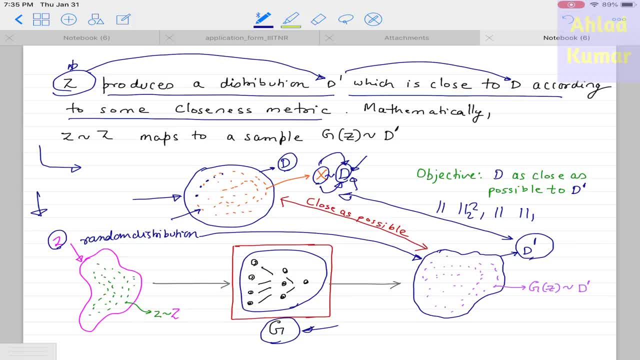 So the target of G is to convert Z, That is, the capital Z, into capital D hat And this capital Z is basically the random distribution And this random distribution is converted into a distribution D hat Which is as close to D. Please note that the samples that are inside this random distribution, capital Z, 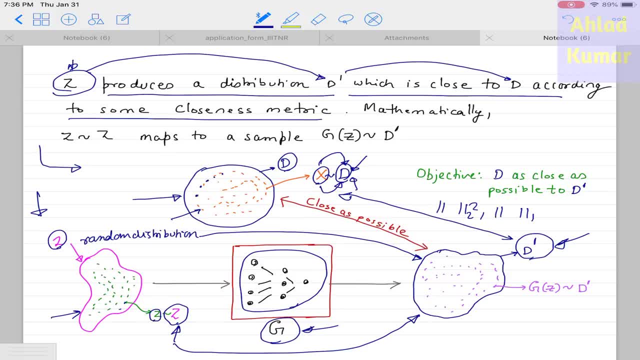 Are represented by small z. And when this samples inside this Random distribution are fed into this Generative model, G Are transformed into G of Z. So all these random variables that are present inside this distribution, That is D hat, Are represented by G of Z. 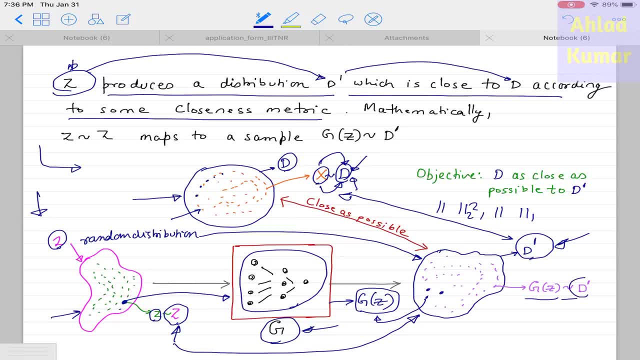 That's why we are writing G of Z Sampled from D hat. So all these samples which are represented by G of Z Are basically generative samples Which are not present in D. What I mean to say is that G of Z 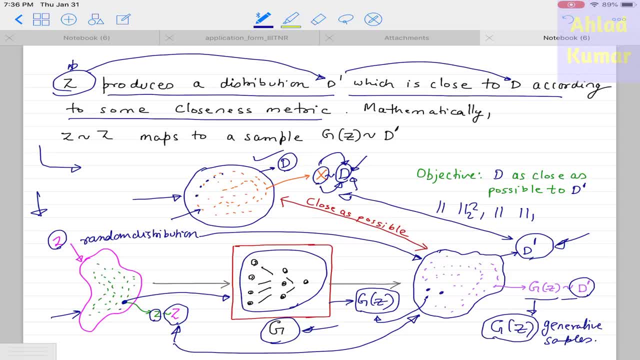 Are also MNIST samples, But these samples are not present in the Already existing MNIST data samples. That is X. So this G of Z Are basically Generative samples which are not present in D, But They follow the same distribution as that of D. 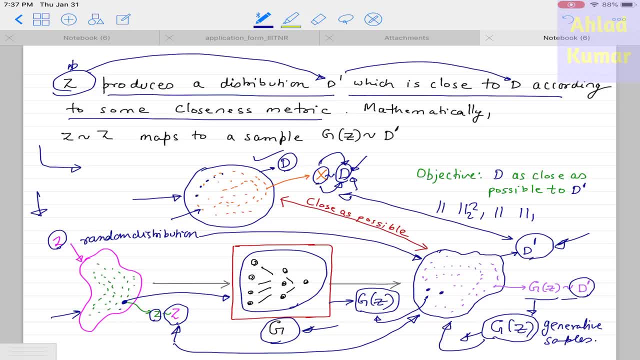 Using this approximate probability distribution, D hat, Which is as close to D. So this is basically the concept Of generative models. So let us see how we can Fit this generative models into Generative adversarial networks and Achieve this target of obtaining. 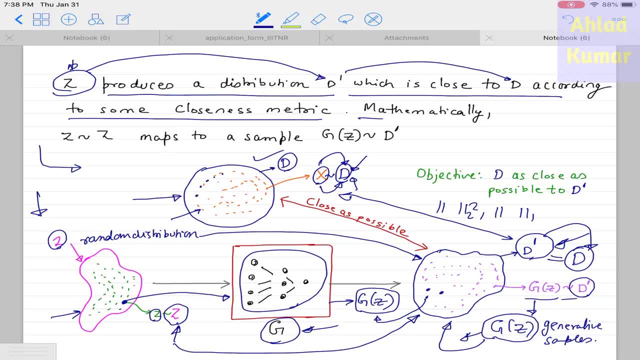 D hat as close to D And mathematically it is represented as this, Which we have already discussed, that is, We are sampling small Z from This capital Z, which is the Random distribution, And what capital G is doing is It is mapping this Z into. 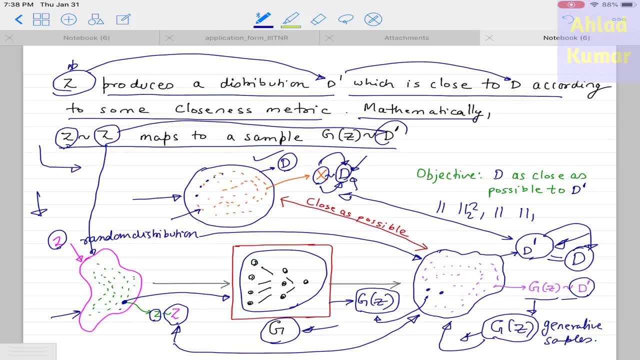 D hat And this D hat is As close as possible to D In terms of L2 non Or L1 non And this G of Z Are basically the generative samples In D hat Which are not present in. 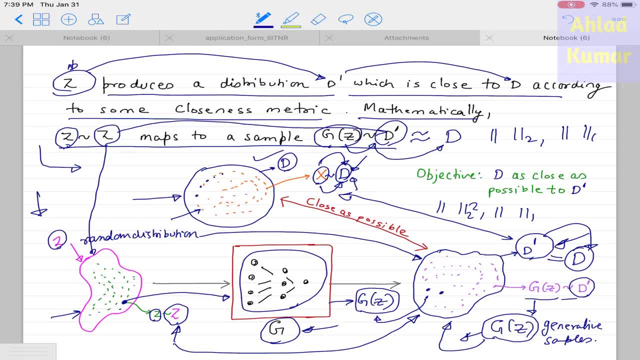 D And they are totally different from The samples that are present in D, But They follow the same distribution as that of D, Because D hat is Close to D In terms of Some Closeness metric. 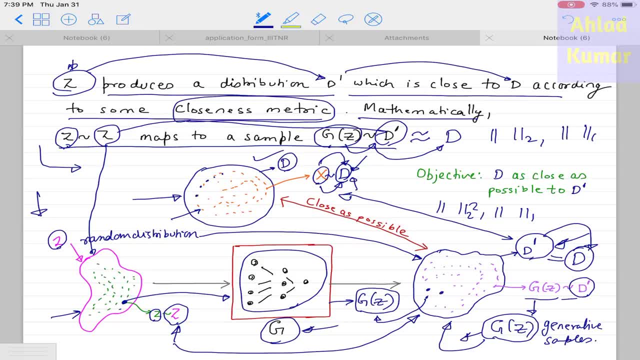 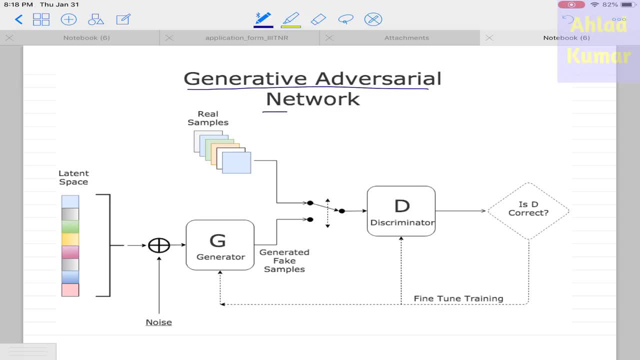 That we will define later. So let's move to the Further details of generative adversarial network. So this is basically the Block diagram for generative adversarial networks that you will find in most of the Literature. So What it is trying to show here is: 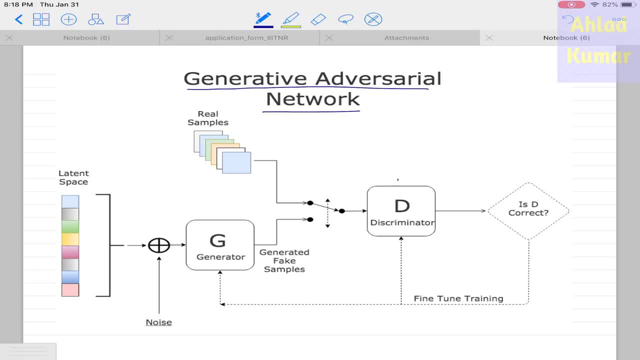 That we have two different models, That are, the discriminative model, which is defined as discriminator, And the generator model that is Defined over here. So the role of the discriminator Is to discriminate Between two different classes And produce the result as. 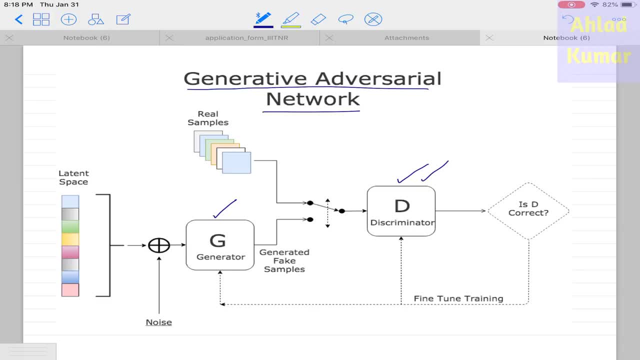 Fake or not fake. That is Zero For fake And one for Not Fake. This is what we have already discussed Here. That is the discriminative model, And this generative model that we have discussed here Is basically represented over. 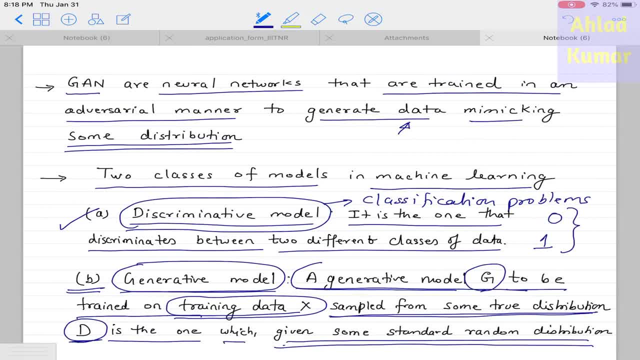 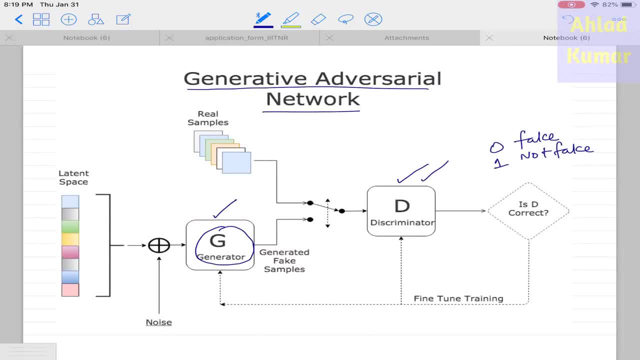 Here. So this generative model is basically Taking the distribution Z From Here To This Generative Model. So This Generative Model From Here And produces A distribution D Hat. 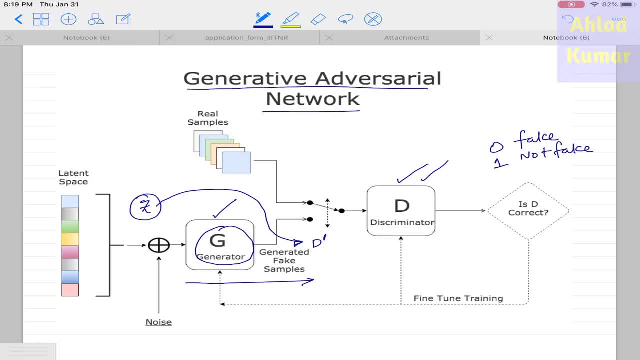 Over here Through this Generator Block And this is the real sample that we are actually talking about And they form the distribution D And the target of the discriminator is to distinguish samples from D And D Hat And produces the output as zero. 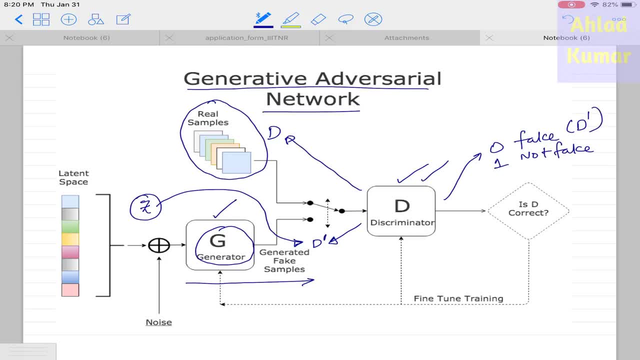 That is fake If it is coming from D Hat, And one Which is not a fake, That is the real one If it is coming from D. So if the decision that is made by the discriminator is wrong, Then a feedback will happen in which 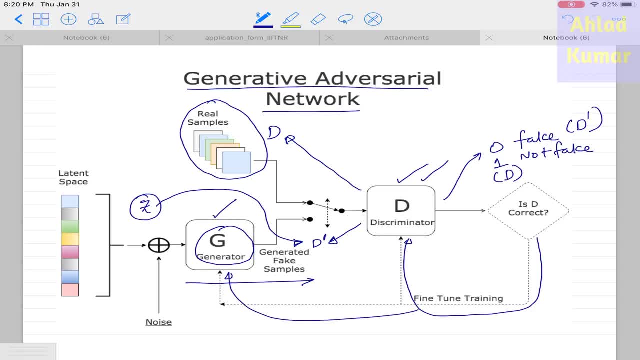 Fine tuning of the discriminator model And fine tuning of the Generator model will be Done In the Back propagation. So this fine tuning is basically Back propagation, Since discriminator and generator are basically neural networks. So fine tuning is Done in. 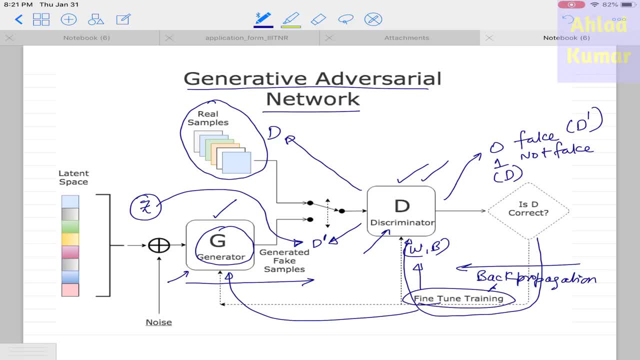 Adjusting the weights And Bias of these Neural Networks. And these latent space are basically the Small Z, Which are Sampled from this Capital Z, Which is the random Distribution, And these real samples are Capital X. 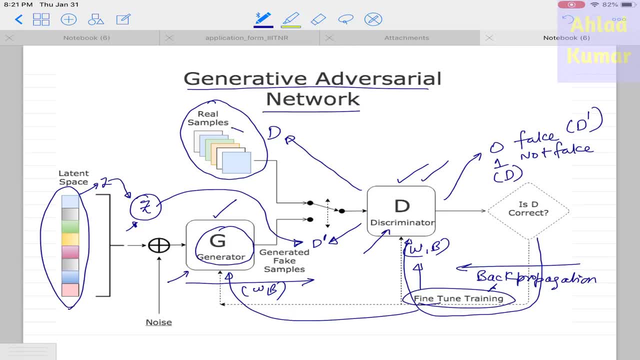 Which we have discussed In our earlier slide. So this is basically the overall concept of Generative, Generative adversarial network. So in this lecture, what we will do is We will be doing a case study on the MNIST. 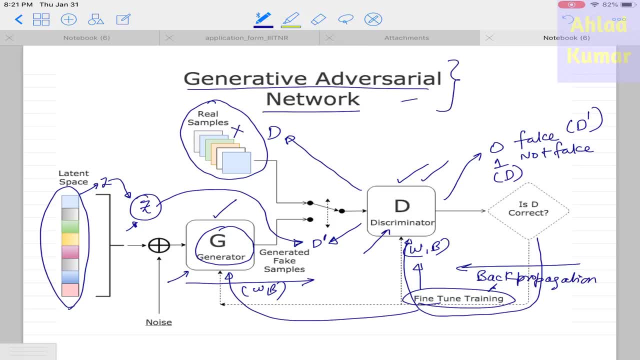 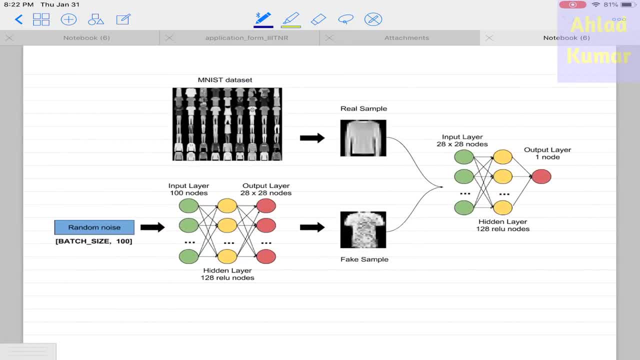 Network Will be represented If we are dealing with MNIST Fashion data set. So this is basically the Internal Representation of Generative adversarial network In case of Fashion data set. Here you can see That we have this. 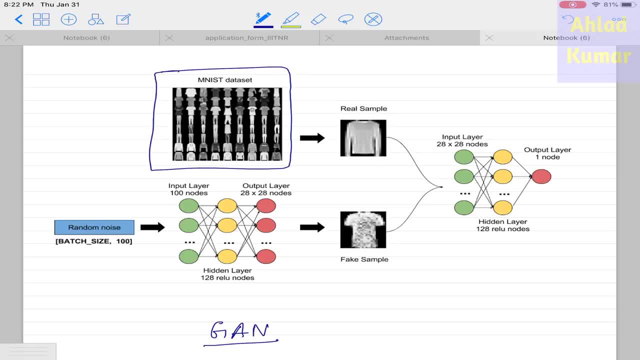 MNIST Data set. This MNIST data set Basically forming a distribution Which is Capital D, And all these Images Which are Present MNIST fashion data set are represented by the random variable x and this random variable. 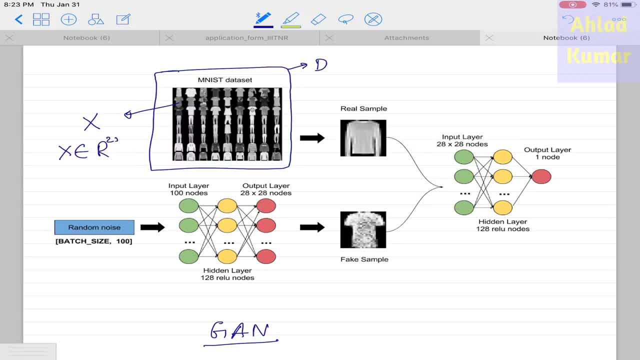 x is basically of dimension 28 x 28, and this is one of the instance of this random variable which is represented by small x, and this is sampled from this unknown distribution that we want to approximate, that is, capital D, and this is basically the generator network which. 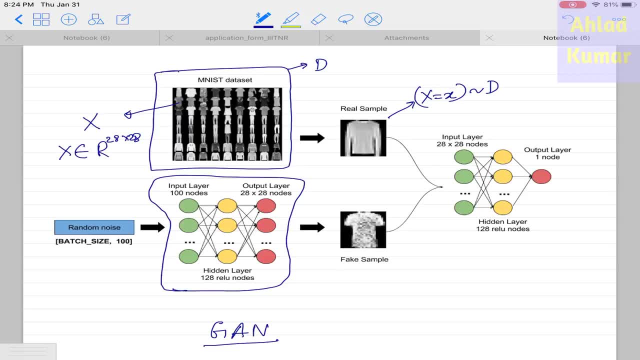 is represented in terms of neurons or the neural network, and this we call as G. so what is the role of G? the role of G is to transform this random variable sampled from this capital Z into G of Z, which is represented by this fake sample actually sampled from some approximate. 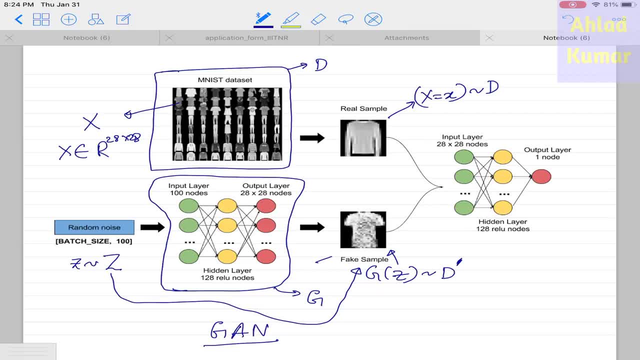 distribution D hat. so this GZ is basically this fake sample and this is our described discriminative model or discriminator, and what it is role. its role is to discriminate between g of z, that is, the fake sample, and the sample that is coming from real data set. 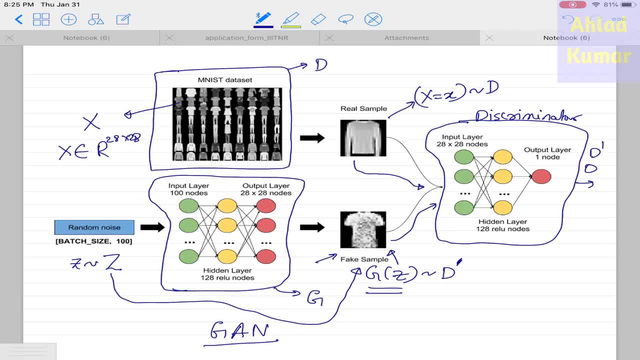 and produces the output zero. if the sample is coming from d, hat and produces the output one. if the sample is coming from d and if it makes a mistake in doing that, then it has to adjust these parameters in the neural network that are available here in terms of weights. 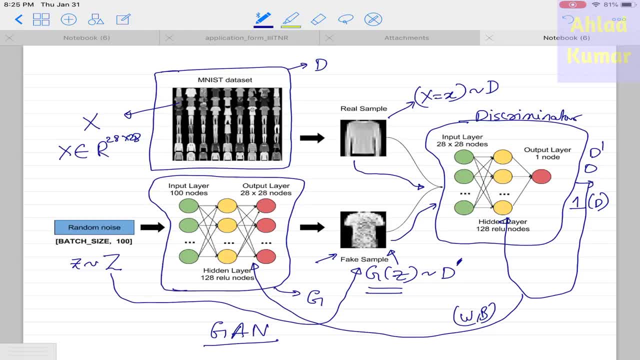 and bias to retrain the system and achieve the desired objective of correctly classifying the images coming from real sample or from the fake sample. so the objective of the discriminator is to distinguish between the real and fake samples and the objective of generator is to produce fake samples which are as close as possible to the real and fake samples. and 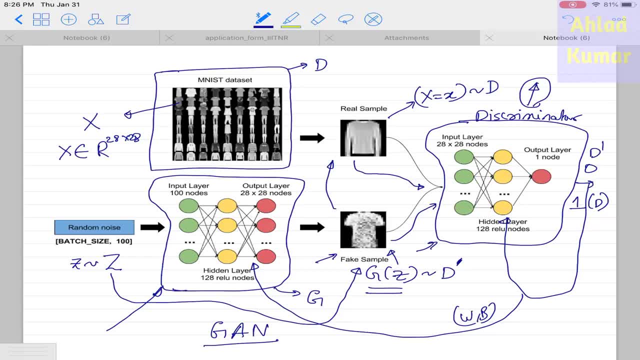 these real samples so that discriminator fails to distinguish between real and the fake sample and produces the output which is neither zero or one for both of these samples. that is, its objective is to make discriminator outputs the value of point five, so in case when its output is point five, the discriminator will fail to discriminate between these real samples. 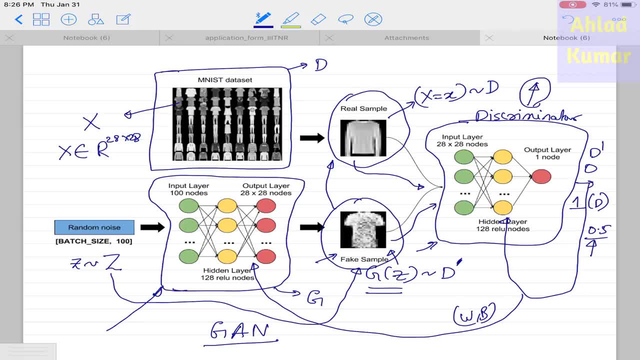 and between these fake samples. the generator objective is to create fake samples that are as close as possible to the real samples. so by doing that means that we are making d hat as close as possible to d. so that is the basic understanding of generative adversarial networks. so lets discuss back. 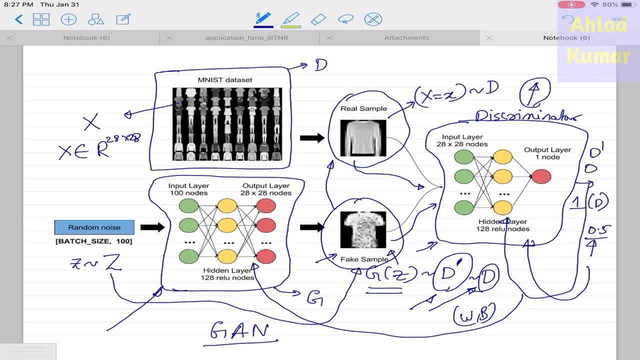 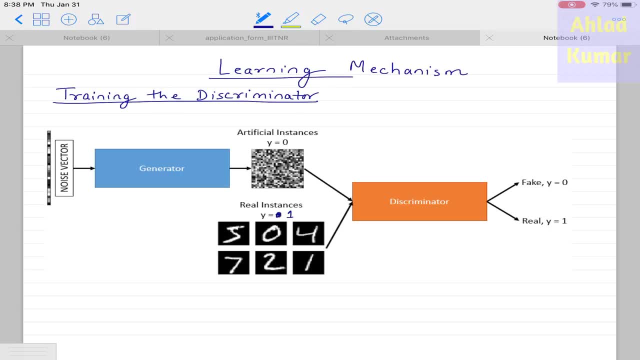 propagation. that is how we will retrain these weights and biases in order to achieve this result in our next slide. so lets discuss the learning mechanism by saying: by saying that learning mechanism means learning the weights and biases of the neural networks that are present in discriminator and generator models, and this learning can be basic. this learning 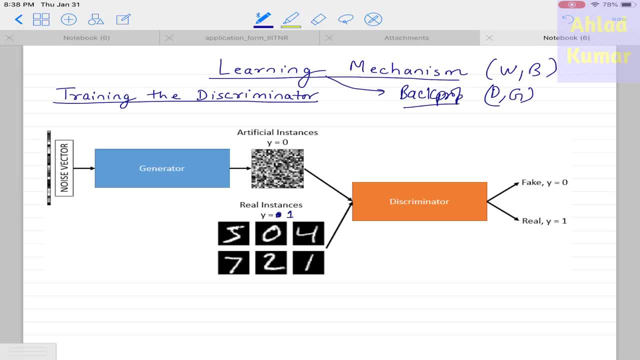 is done using back propagation, so lets discuss that. so the thing is basically. a GAN is composed of a discriminator and a generator, as we have discussed. each of these are held constant while training the other. please note that its important, so we will thus alternate between training the discriminator and the generator. 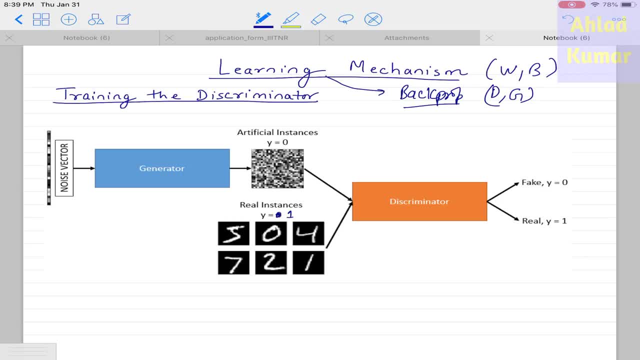 this is done separately. training the discriminator is much easier, so lets look at this first. so the discriminator, as you can see here, has two output nodes, that is, zero and one, and its basically used to distinguish real instances from the artificial instances. artificial instances means the instances that are being produced by this generator network and the real instances. 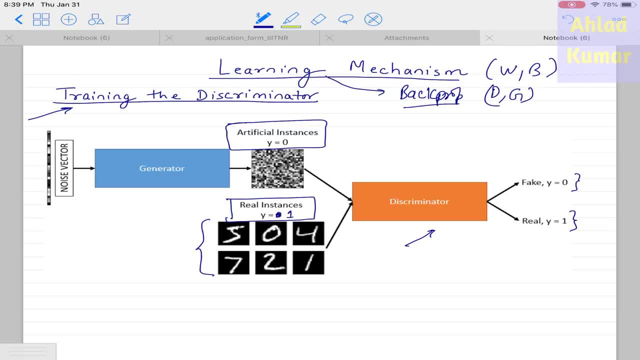 are the instances that are actually obtained from MNIST dataset and basically these instances are sample of this known distribution D. so to train the discriminator is very easy, and the way we do is we feed this noise vector that is present over here into the generator which produces this artificial instance and we label this. 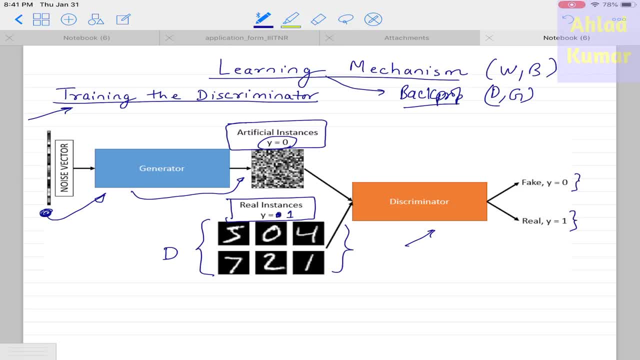 artificial instance as y equal to 0 and along with this we will take the real instances also, which we label as y equal to 1, and we feed these images, that is, the artificial images and the real images, into this discriminating model to distinguish between the fake images, that is the images. 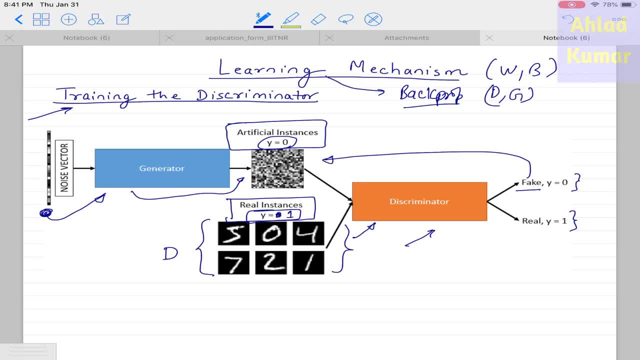 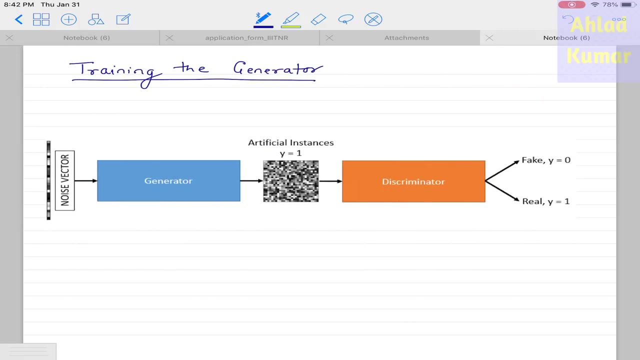 that are coming from artificial instance and between the real images, that is, the images coming from real dataset. so we can see that discriminator is trained exactly in the same way as a basic classification task done by CNN, having two different output nodes. so its basically a simple classification task. now the next task is to train the generator model. 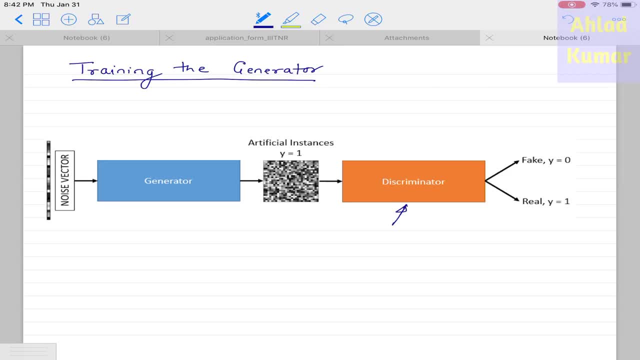 so when we train the generator, we will keep the discriminator fix, that is, we will not train its weights and biases. this is important. so the reason for doing that is we do not want our discriminator to become too strong to ever beat. so once we fix the discriminating, 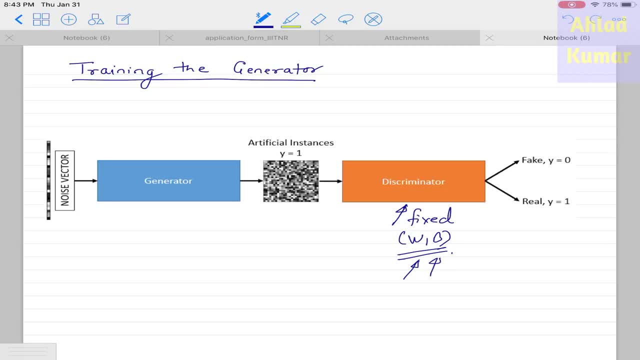 model. so in case of training the generator, what will happen is we will again create this noise instance that is small, z, taken from the distribution capital Z, and convert it into a artificial instance, and we want our discriminator to get fooled by this image and produce the 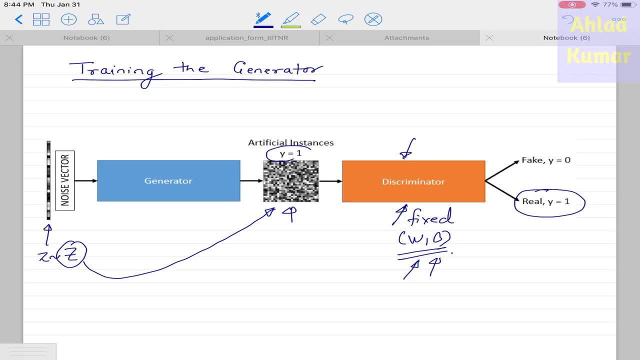 output as 1. so that's why we are labeling here this as y equal to 1, though it's a artificial instance. so in training the generator, what we are trying to do is we are making generator smart enough so that it can fool the discriminator and produces output as 1 if it fails to do. 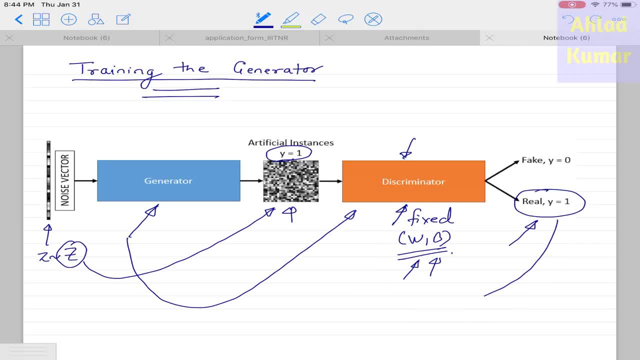 that then the error is back propagated and the weights and bias of this generator network are adjusted so that it becomes more intelligent and tries to produce this artificial instances as close as possible to the MNIST data set. and once it is able to achieve that target, then the discriminating model will.